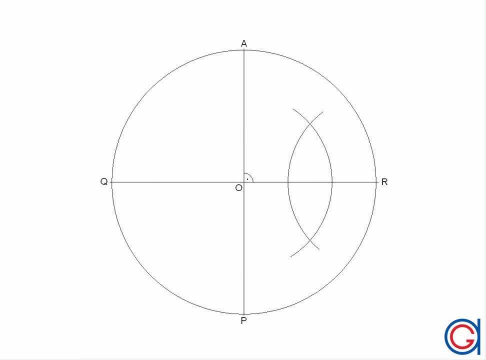 These two arcs intersect at two points, and now we will join these two points. and where it cuts the radius OR, this will be the midpoint M of the radius. So now, with our compass centered on M and radius MA, we scribe an arc to the left. 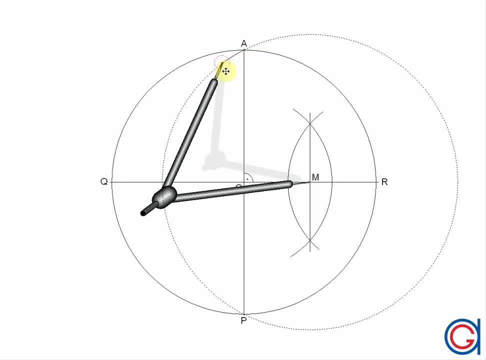 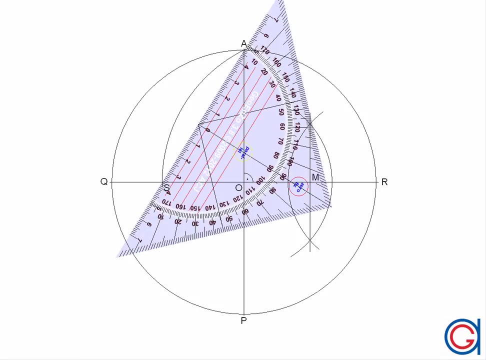 until it cuts our horizontal diameter Q, OR We will call this point S. So now we join point S to point A with a thicker line, and this line, segment SA, will be the length L of one side of our pentagon that we want to draw. So the next step is: with our compass, we want to 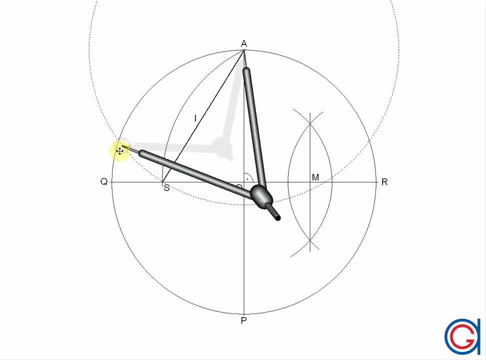 transport our length L onto our circumference five times, starting at point A. So, as you can see, we scribe our first point. Now, setting our compass on this point, we scribe our second point. Again. following this process, we set our compass on our third point and scribe: 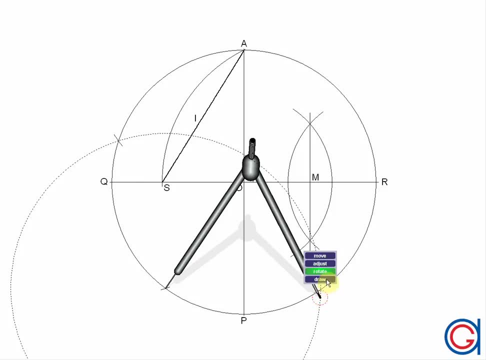 our fourth And again setting our compass on point four. we scribe our next point And, finally, if we are doing everything with precision and accuracy, our final arc should cut exactly on point A. So we are going to set our compass on point B and again setting our compass on point. 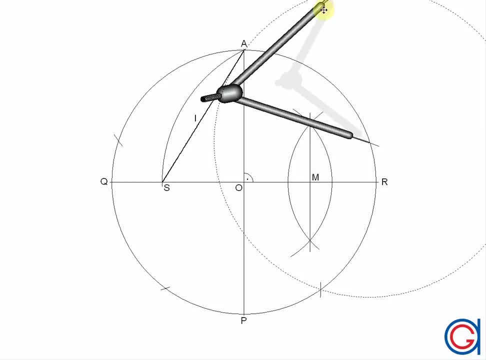 four. And finally, if we are doing everything with precision and accuracy, our final arc should cut exactly on point A, as can be seen here in the video. So the next step is to name the final four vertices of our pentagon: B, C, D and E. 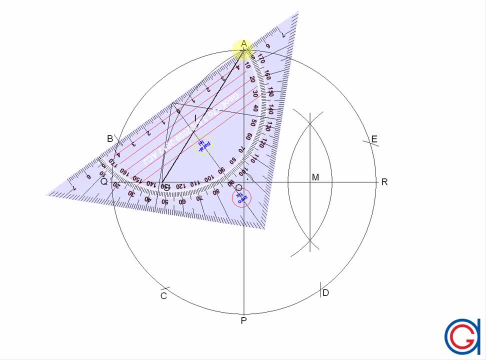 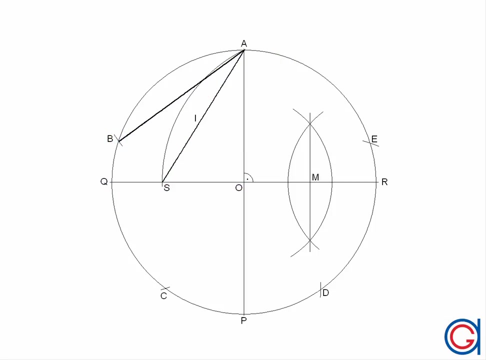 And finally, with a thicker line, we will join our vertices A to B. And finally, with a thicker line, we will join our vertices B to C. And finally, with a thicker line, we will join our vertices B to C.